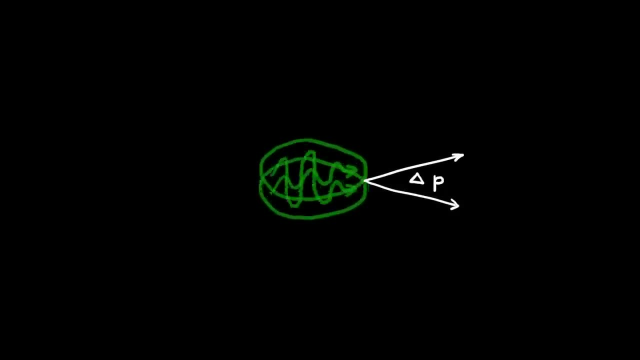 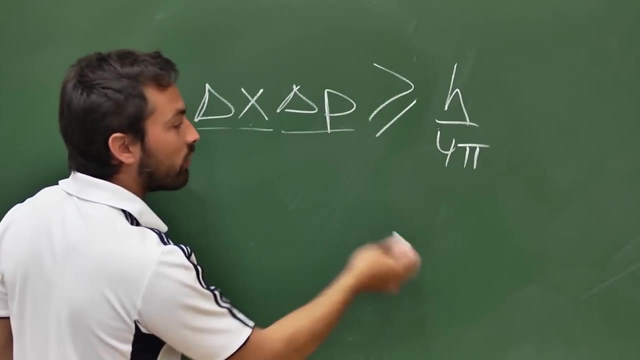 So delta x is the uncertainty in position and delta p is the uncertainty in the momentum. Now, if you multiply those two quantities together, they must always be greater than or equal to h on 4 pi. Now h is Planck's constant. 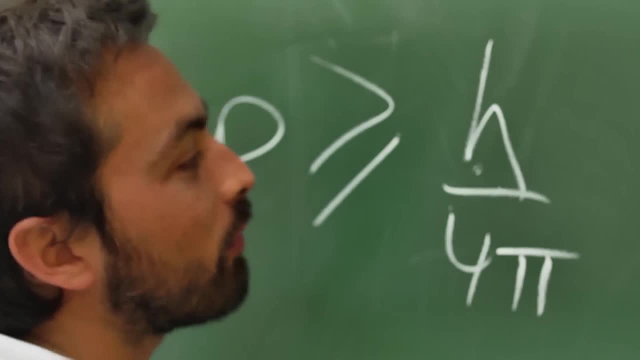 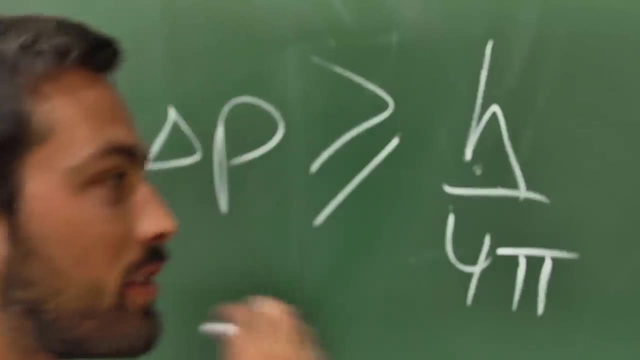 And that deserves a video all to itself, like this one by 60 Symbols, But for our purposes it's just a very small number. So in our everyday lives we don't come up against this uncertainty relation, because everything is much, much bigger than h. 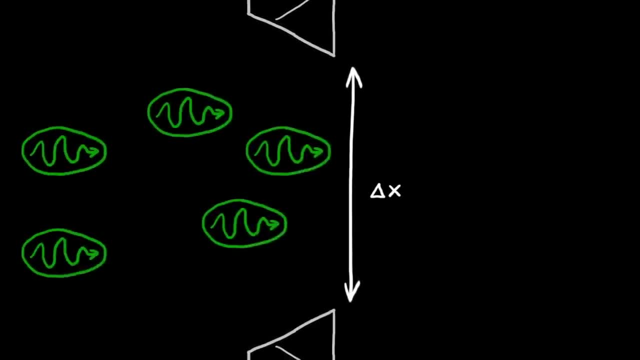 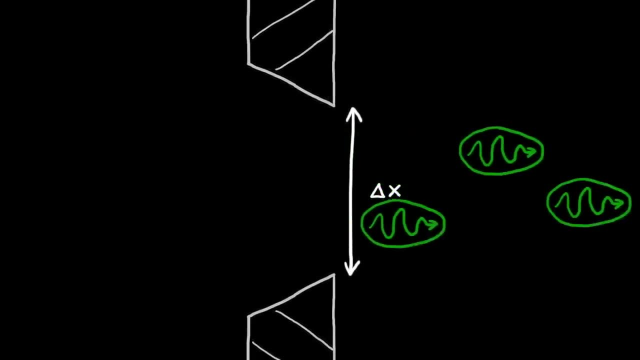 But as we narrowed the slit we were decreasing delta x for those photons. So we were getting more and more precise about where the photons were passing through that slit. And at a certain point you come to this limit, so that if you narrow this any further, 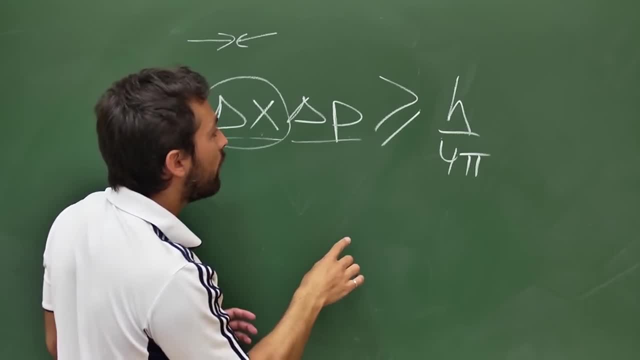 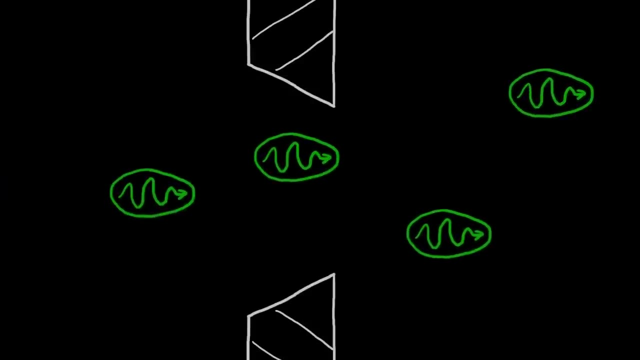 you're going to break this uncertainty relationship. So what needs to happen is the uncertainty in momentum needs to go up. I should specify: this is uncertainty in momentum in the x direction, in the horizontal direction. So if before photons were going perfectly straight? 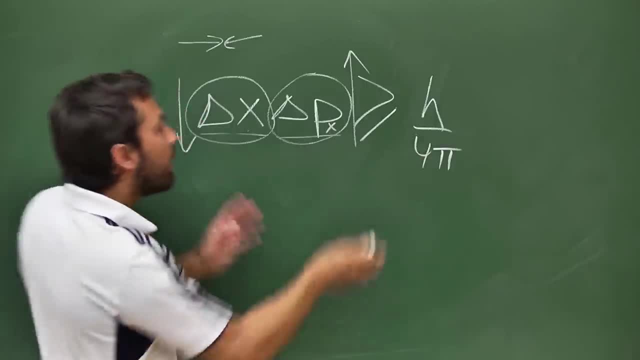 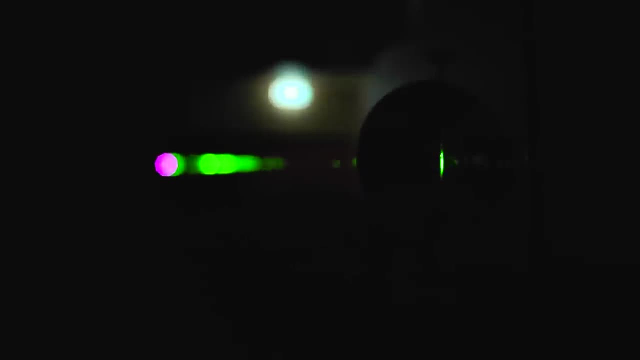 now they must veer off to the left or to the right to ensure that we don't break Heisenberg's uncertainty relation. And the more you decrease your uncertainty in position, the more narrow you make that slit, the more the uncertainty in momentum has to go up. 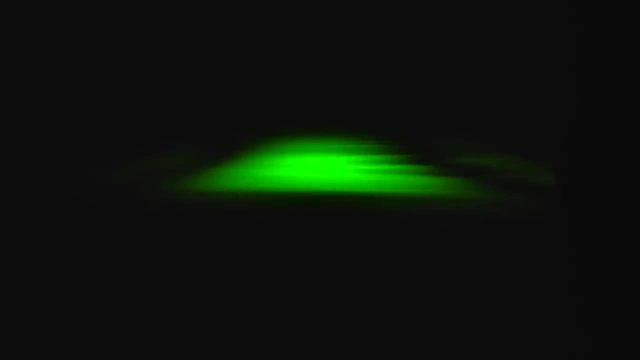 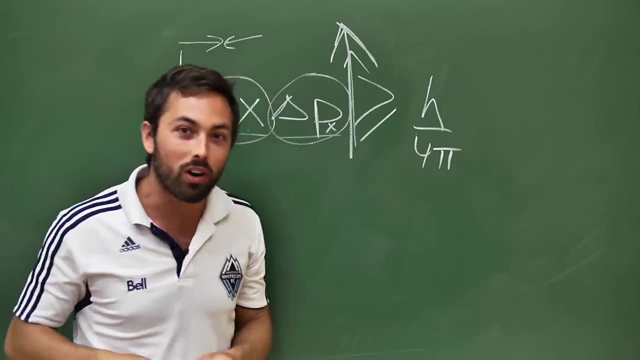 And so if these photons are going to the left and the right, that's going to produce a much wider beam. It's really, really non-intuitive, but it's the way the world works. I don't know what that is. It must be the sun playing tricks with my mind. 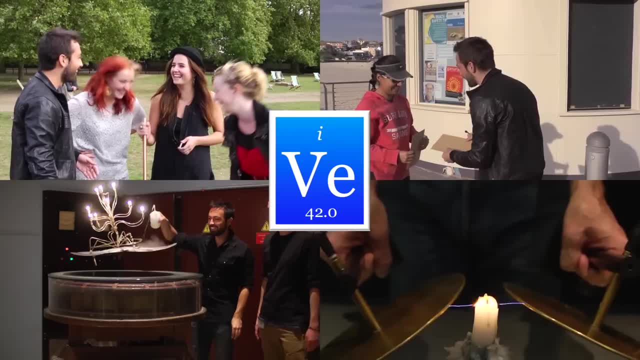 I think it's the powers of the universe. What about here's really going to test you right? I don't know. I don't know why I said that. Well, this is before you said it. It's only a few blocks from here. 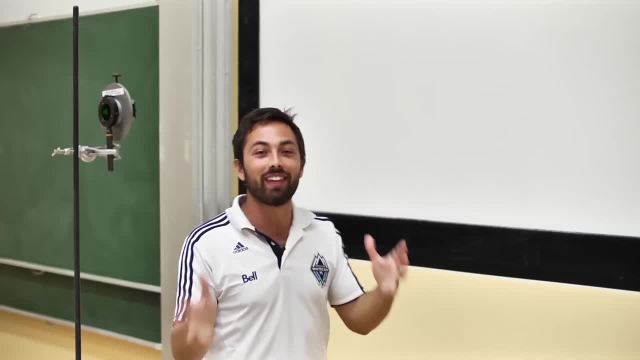 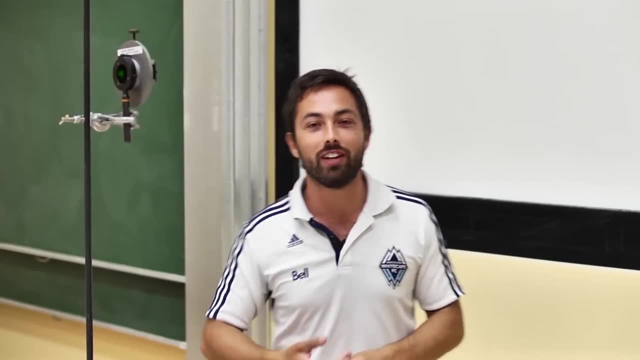 So what do you expect? that we'll see every day. I've got to say a big thank you to Professor Walter Lewin at MIT. He inspired me to make this video- And I also have to say a big thanks to the University of Sydney. 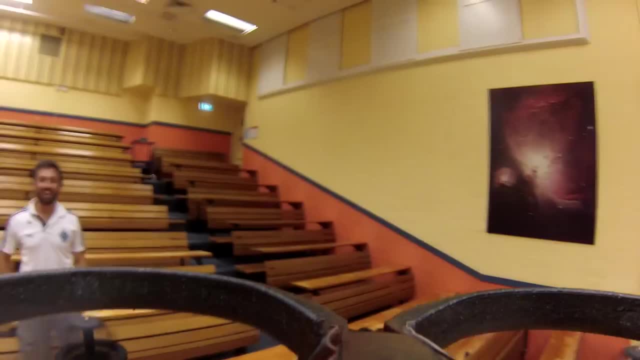 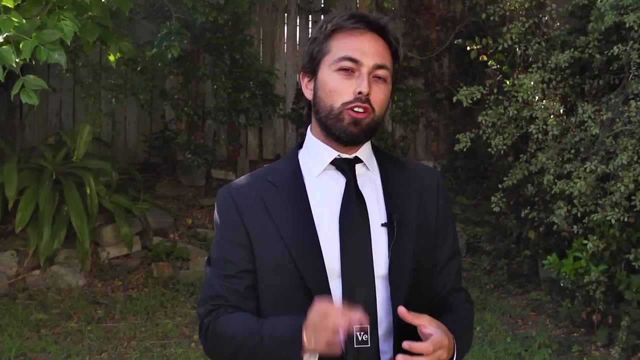 for letting me use their equipment, and especially to Tom and Ralph for letting me set this all up. Oh, and just one more thing. I should point out that this explanation of the experiment is slightly controversial, at least in that Henry from MinutePhysics and I